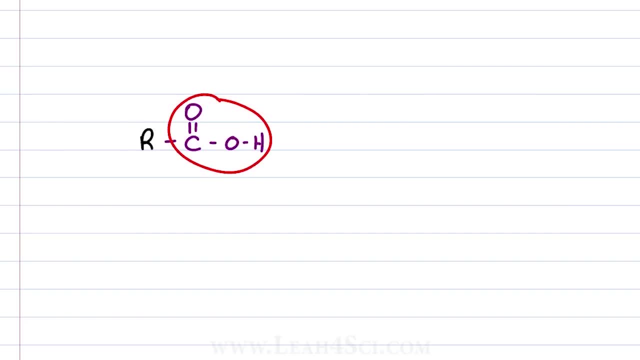 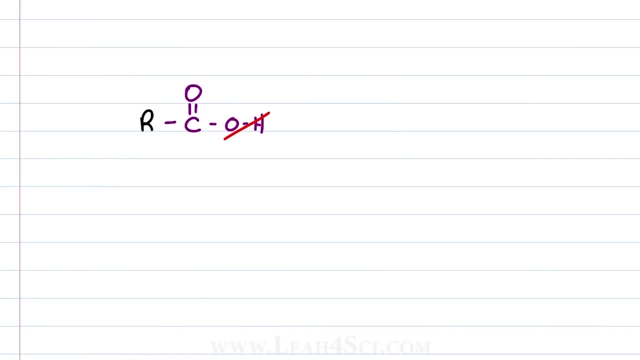 hydroxy, but it's not an alcohol, because together they form one functional group called the carboxylic acid. If we remove that OH and replace it with different groups, we get a derivative of carboxylic acid, because we're deriving it from the carboxylic acid and we're 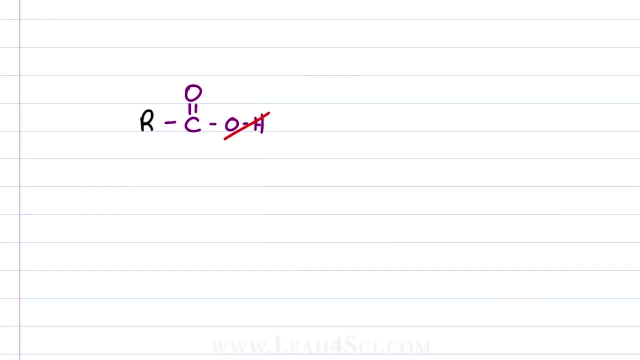 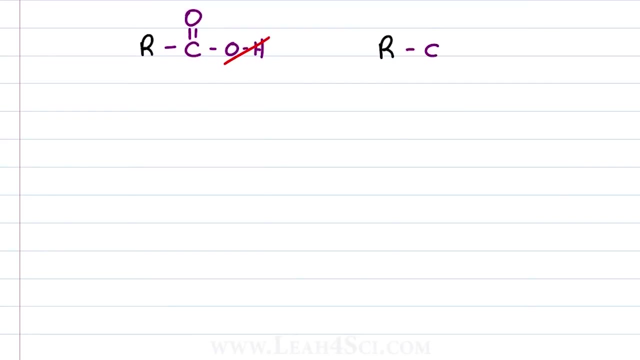 deriving it from the carboxylic acid molecule, and this leads to a whole new set of reactions that you can use in synthesis. Some professors will refer to the derivative as the carboxylic acid parent, with either a Y or a Z here, where that Y or Z represents the new group which 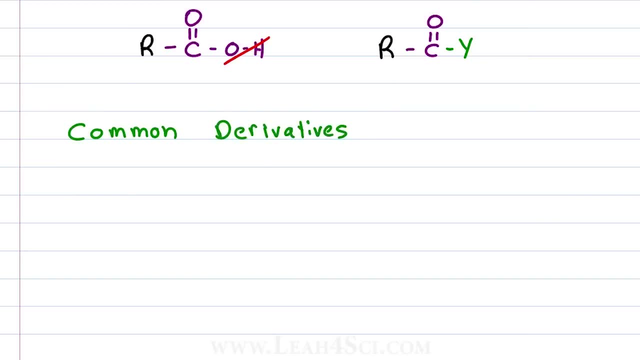 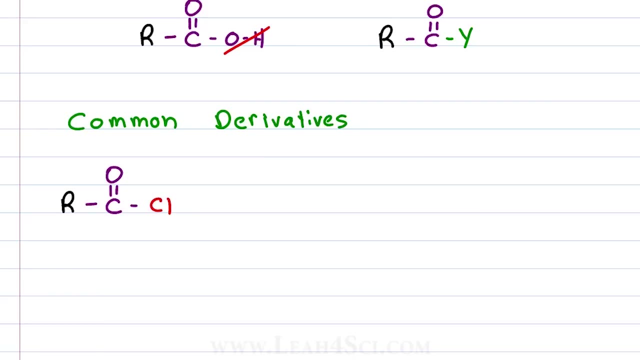 gives you the specific type of derivative. Let's look at some common derivatives, from most to least reactive. If I replace the OH with a halogen, for example chlorine, I'm going to have a carbon double bound to an oxygen. that will give me an acid halide as 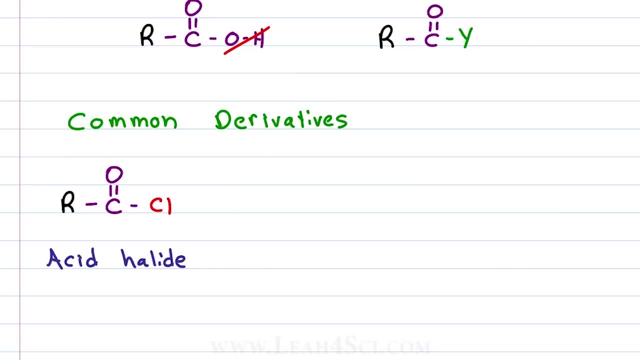 the general class, or an acid chloride for the specific molecule. This is also called an acyl chloride or an acyl halide, If I replace the OH with what looks like another carboxylic acid without the hydrogen. so we'll just have this portion here, giving us an oxygen, a carbon. 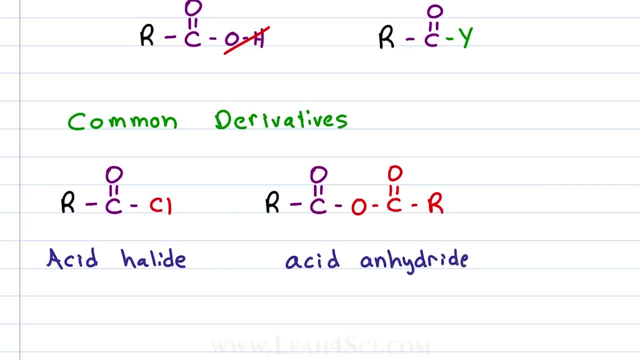 double bound to an oxygen, and then a second R group, Or simply anhydride. If you think about it, if we split the molecule in half and add in a water OH and another H for H2O, that would give me two carboxylic acids. so we have the. 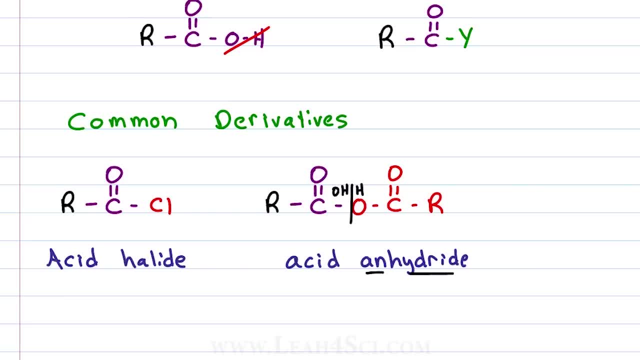 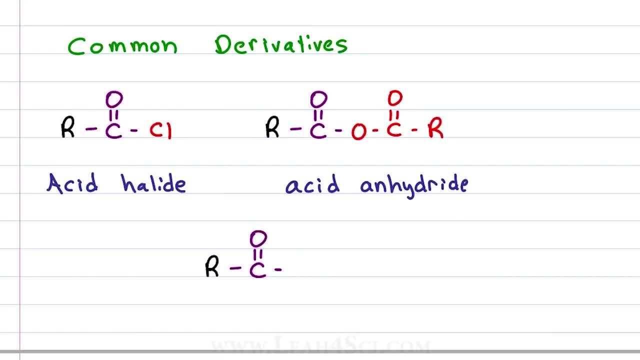 acid without water, anhydride without water- that's how we get the acid anhydride derivative. If we replace the OH with an OR group- and it's not just the H that we're replacing with an R- Let's say your group got swapped for a brand new oxygen and R group, Then I get what's. 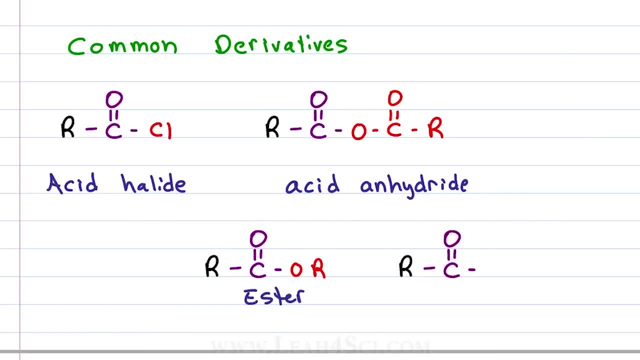 called an ester. and if I replace the OH with a nitrogen, for example NH2, or we can have NHR or NR2, these are just different substituted nitrogens- we get what's called an amide or amide. Let's face it, your professor is not just sticking to the common derivatives. you might 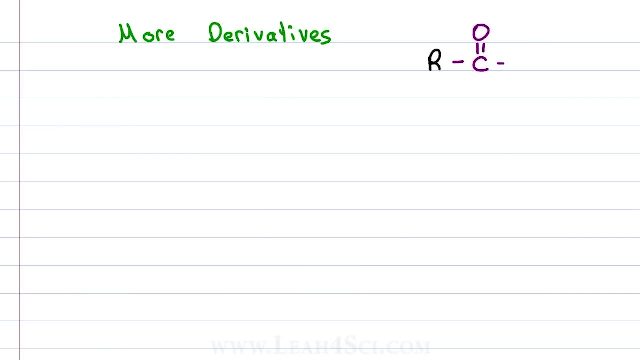 also see some of these less common molecules. Let's face it, your professor is not just sticking to the common derivatives. you might also see some of these less common molecules. As a reminder, a carboxylic acid starts out with a carbon double bound to an oxygen. 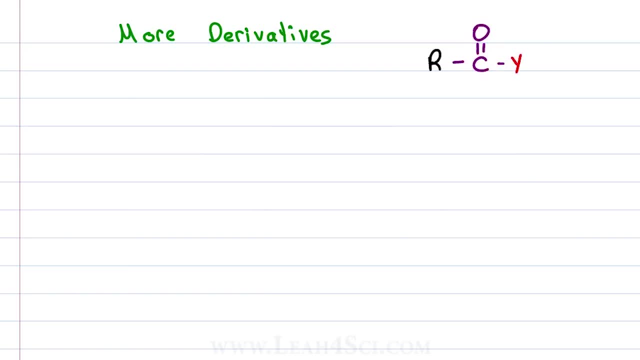 So if we replace the Y, we get a derivative, But recognize that what we have here is the carbon bound 1,, 2,, 3 times. So if we have carbon bound 3 times to something else, that would still qualify as a carboxylic acid derivative. For example, if I remove that oxygen and instead 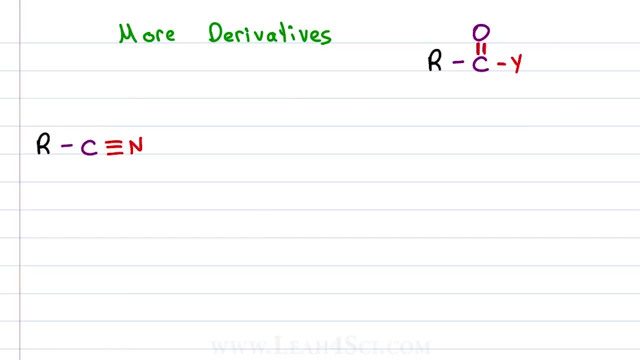 oxygen and instead have three bonds to a nitrogen. that gives me the nitrile derivative And finally cyclic derivatives, which are just cyclic versions of their linear counterparts. but for some reason seeing that ring scares students. Don't let this scare you. If I have a ring with a carbonyl bound to an oxygen and then the ring happens to close, 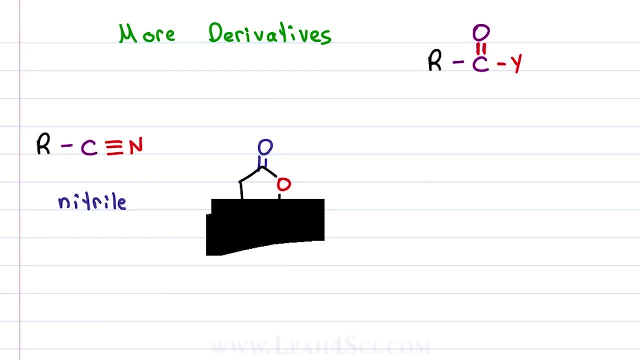 in on itself. doesn't this just look like an ester where we have an R group here and here as two separate chains? This gives us a cyclic ester, which is also called a lactone, If I have the same structure with a nitrogen instead of an oxygen, along with a hydrogen. 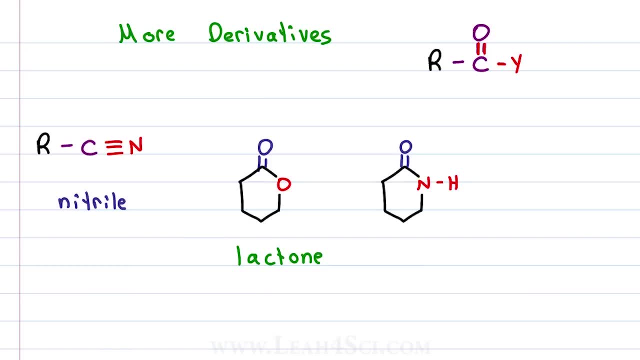 because nitrogen needs three bonds where oxygen needs two. you should recognize this as a cyclic amide. If we take off the bottom, This is simply carbon chain number one for the carboxylic acid, and this would be a second carbon chain for a substituted amide, but the two chains happen to be connected. 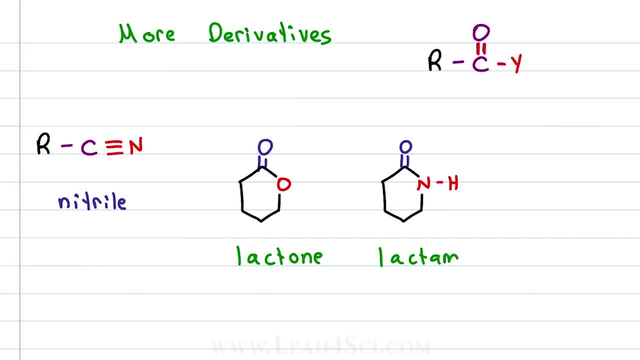 The cyclic amide is also called a lactam, and this is where students get confused The way I remember the difference is: the lactone has the extra O for the cyclic ester and the lactam is the cyclic amide, which tells me it has a nitrogen. 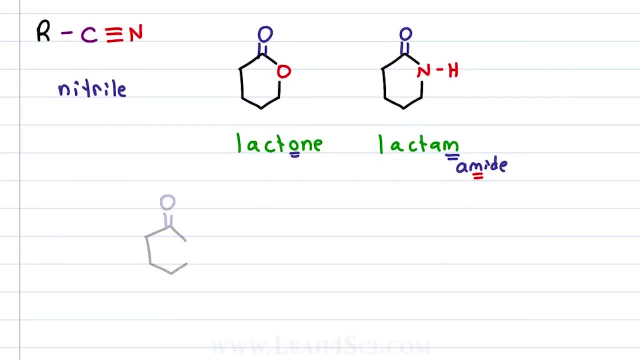 Okay, You may also come across something that looks like this: It's a cyclic structure with an oxygen in the middle, but another carbonyl. You should recognize this as a sideways acid anhydride and in fact it's just a cyclic. 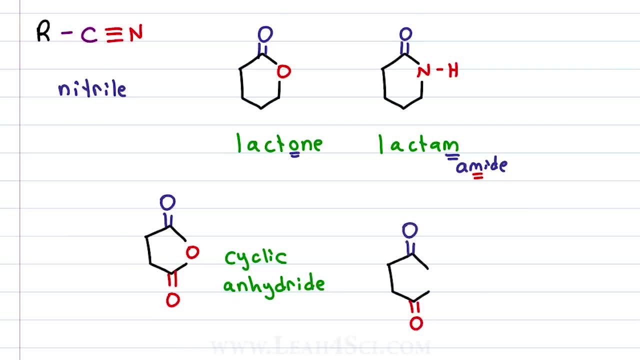 anhydride. and if I take that same cyclic anhydride but replace the oxygen with a nitrogen, I don't get a cyclic amide because the linear version would be called an imid. Remember, An imid is when you have a carbonyl on either side of a nitrogen, so this would simply be. 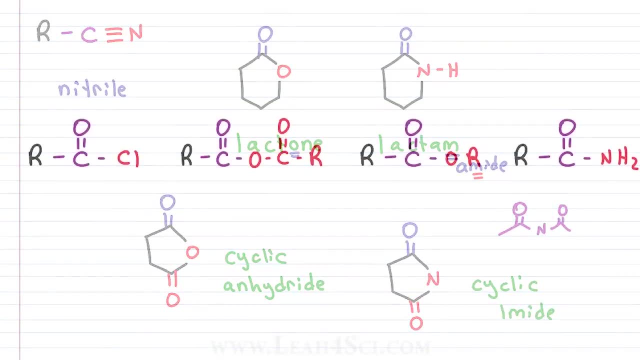 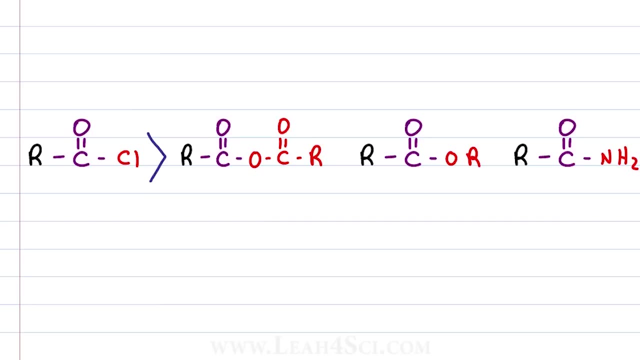 a cyclic imid. When looking at reactions of carboxylic acid derivatives, it's important to remember that the acid halide is most reactive, then the acid anhydride, then the ester, and least reactive is the amide. 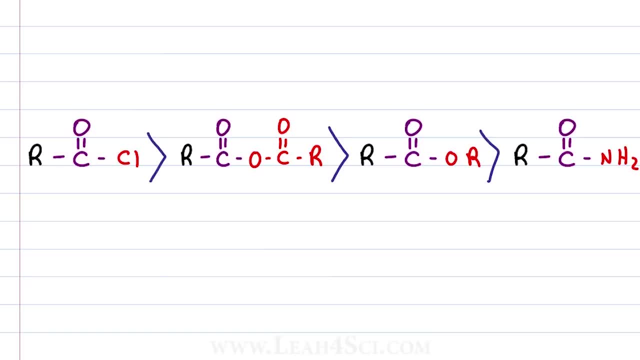 As a reminder, all of these are listed out on the carboxylic acid derivative cheat sheet, which is linked below. When you hear most reactive, recognize that it's going to react the fastest, has the best leaving group and therefore is least stable, as is, but most stable when the leaving group 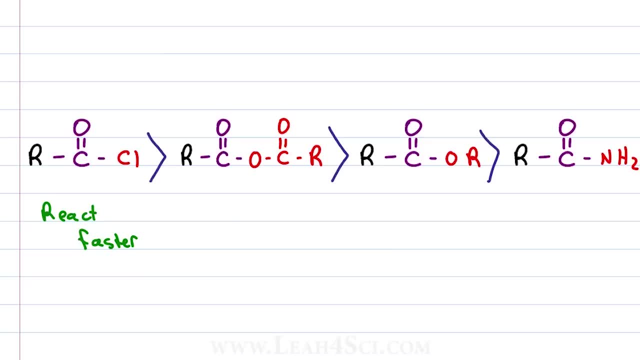 departs. The amide being the least reactive, tells us that it reacts slower, it has a bad leaving group and therefore is least stable when you kick it out. This is important to recognize because it's very easy to make a less reactive derivative. 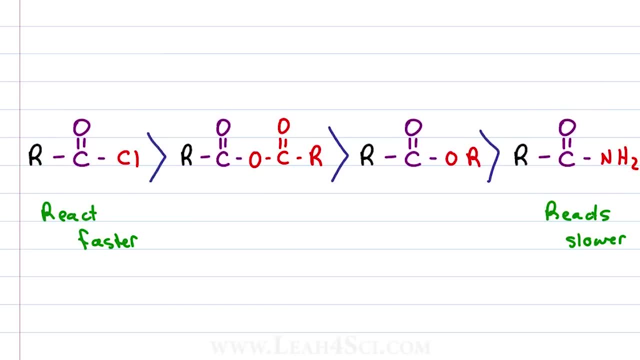 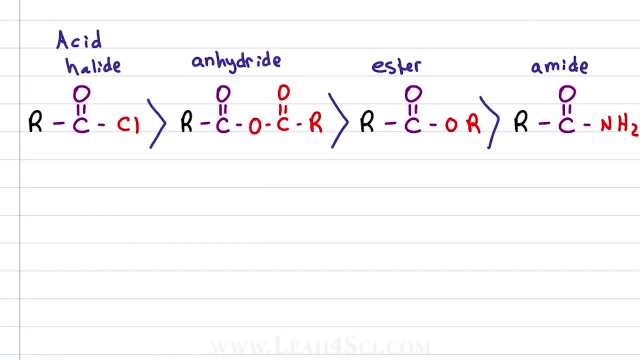 a more reactive derivative, but it's going to take more extreme conditions to go from something less reactive to something more reactive, because it wants to go in that direction. This video is just an overview of the reaction, so let's see how you go from one to the next. 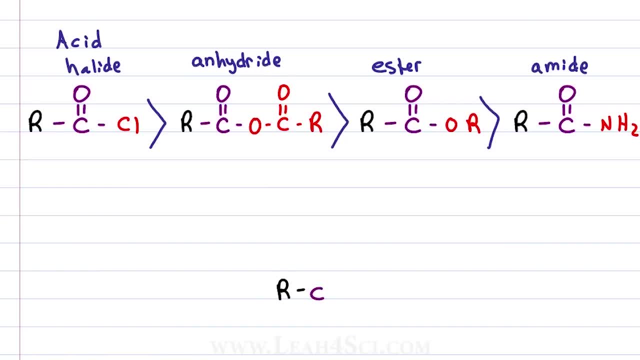 In doing so, we can't forget the carboxylic acid, because as a derivative, we also need to know how to go from a carboxy to any of the derivatives. A carboxylic acid will form an acid halide. 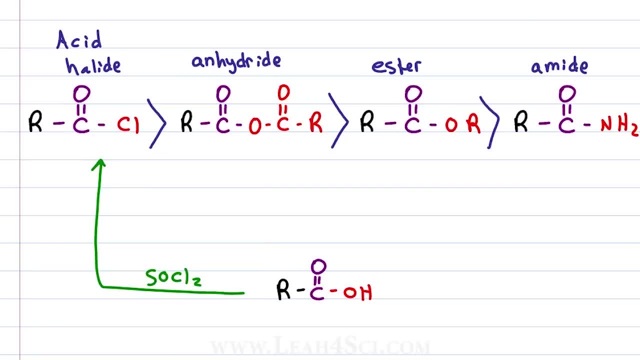 When reacted with something like SOCl2, which makes the OH a good leaving group and brings us a source of chlorine. To go from a carboxylic acid to an acid anhydride you need to detour. First you make your acid halide, which is very reactive. then you simply react the acid halide. 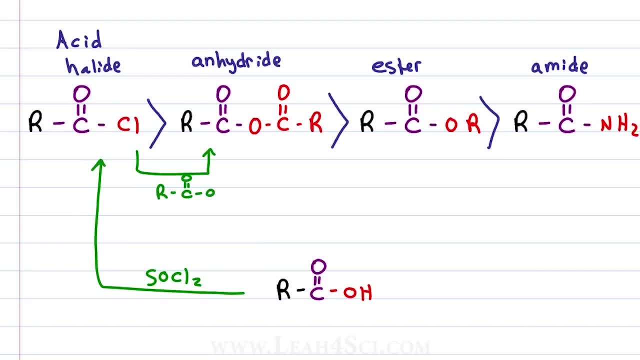 with a carboxylate or a negative deprotonated carboxylic acid, which will kick out the chlorine and give us the acid anhydride. The carboxylic acid is a very reactive derivative. The carboxylic acid is very close to the reactivity of an ester. 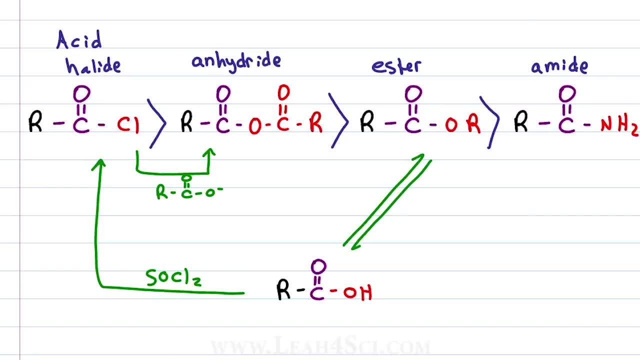 That means it's very easy to go back and forth between the two, depending on the reaction conditions. For example, putting this in an acid catalyst, the more of that derivative component that you have in solution, the more of the reaction favors that direction. 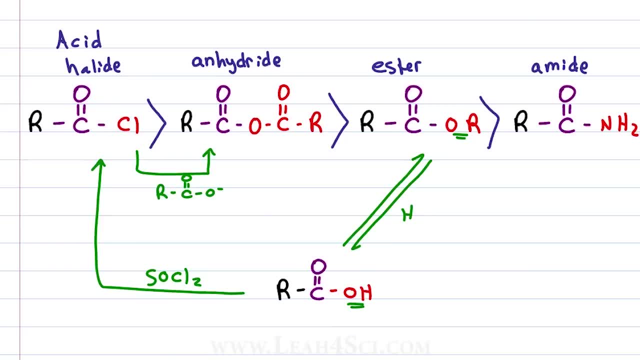 To go from an ester to a carboxylic acid, we just need a whole lot of water, which is the conjugate acid of the OH group. So we'll show H3O plus or water and an acid. So we'll show H3O plus or water and an acid. 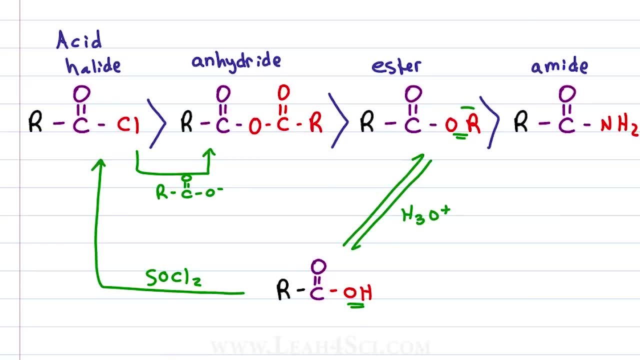 To go from the carboxylic acid to ester. we just need a lot of OR. So we put an alcohol solution with an acid catalyst To go from the carboxylic acid to the amide. we react this in ammonia, but it doesn't stop. 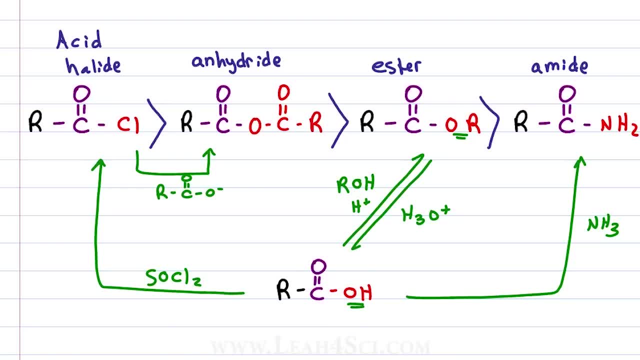 there Another way to make any of the derivatives, especially if you're stuck on an exam synthesis question and you don't remember the exact conditions. best way to do it go from the carboxylic acid to the acid halide. How does this work? 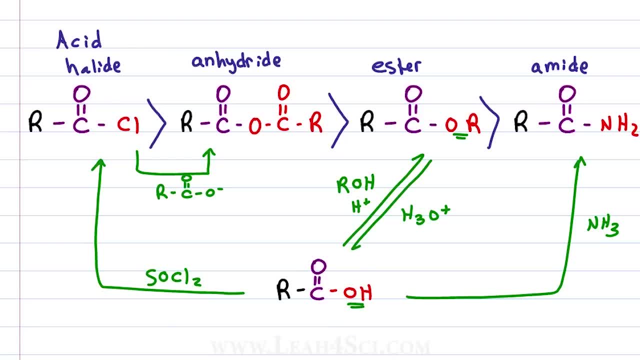 halide. Make sure you know the SOCl2 and then just take that red portion, the derivative portion, react it with the acid halide and you're good to go. We've already shown an acid halide to an acid anhydride using a carboxylate, which is the. 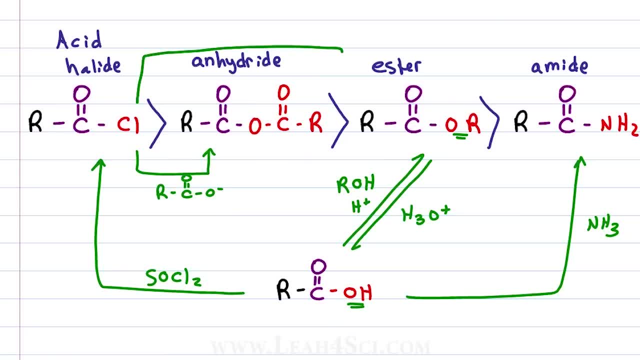 red portion of the anhydride. If I react the acid halide with an alcohol which gives us the OR portion, I'll get an ester, And if I react the acid halide with ammonia or an amine, I will get an amide. 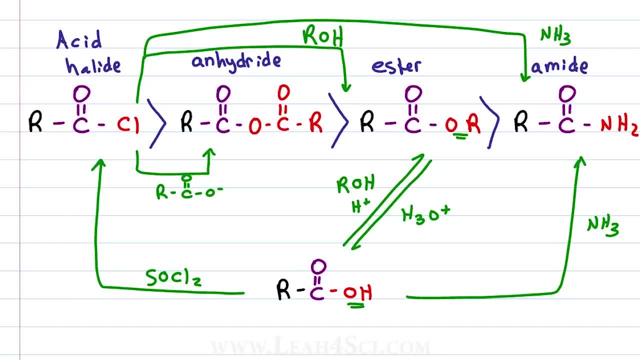 Ammonia would give us just the NH2 amide, but an amine would give us a substituted amide which would be NRH or NR2. but it doesn't stop there. Anytime you want to make something more reactive, the less reactive group will get you there. 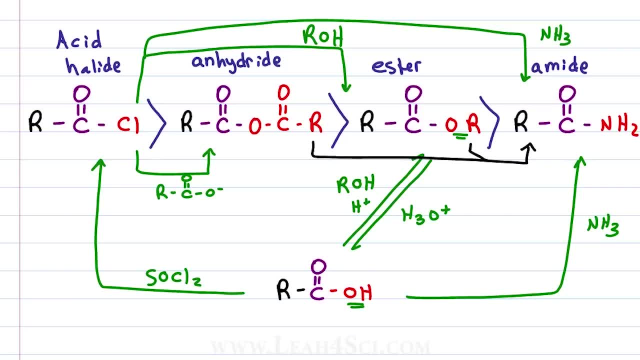 This means the anhydride will react with something like ammonia. So if I react with an acid halide, it will react with an acid halide, and so will the ester. Finally, the last thing you should look at is how to go back to the carboxylic acid from.